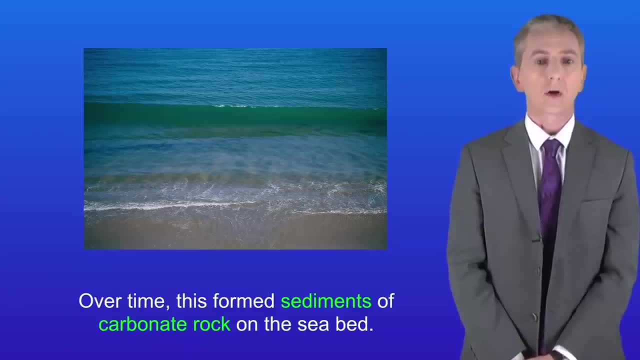 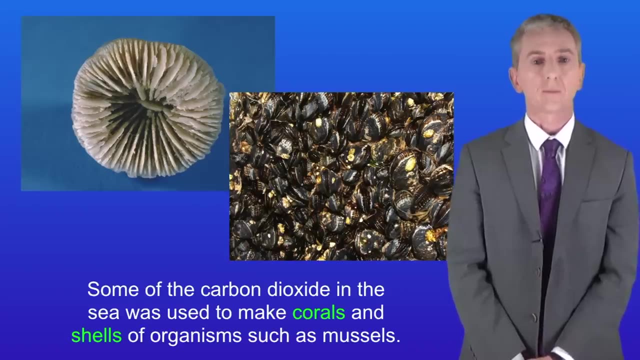 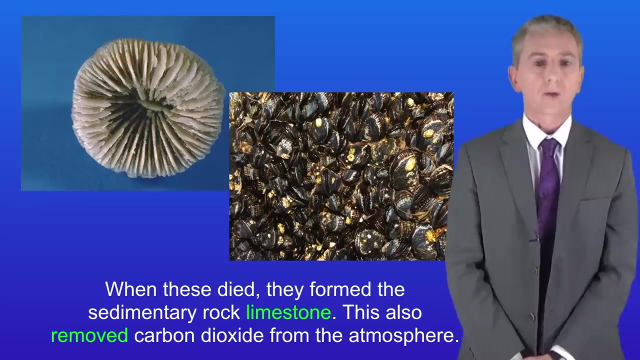 over time, this formed sediments of carbon dioxide. So in the early atmosphere, the atmosphere contained very little oxygen. So, as we can see, the level of carbon dioxide in the early atmosphere began to fall. But where did the oxygen come from? Well, around 2.7 billion years ago, photosynthetic algae. 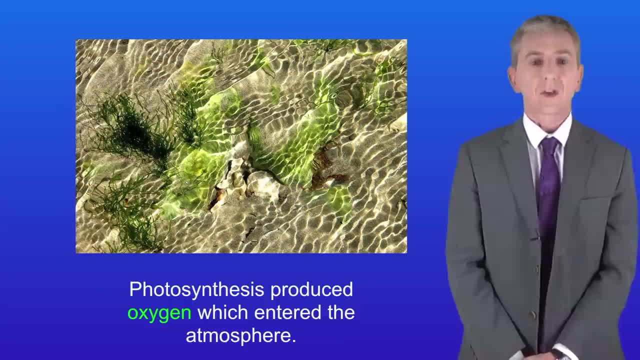 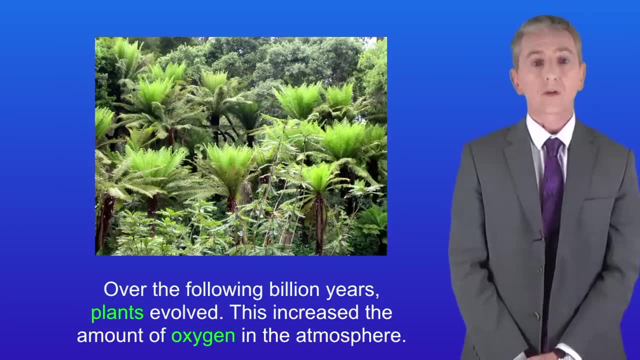 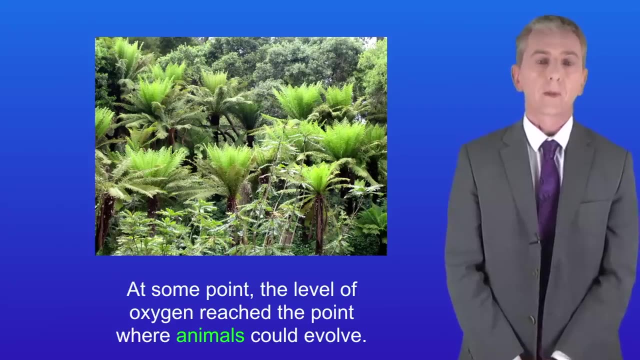 first evolved in the ocean. Photosynthesis produced oxygen which entered the atmosphere. Over the following billion years, plants evolved and this increased the amount of oxygen in the atmosphere. At some point, the level of oxygen reached the point where animals could evolve. I'm showing you. 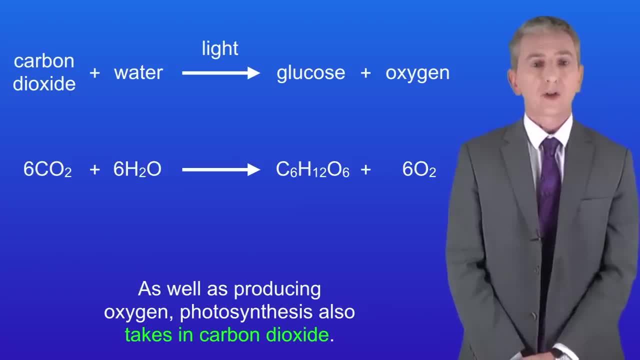 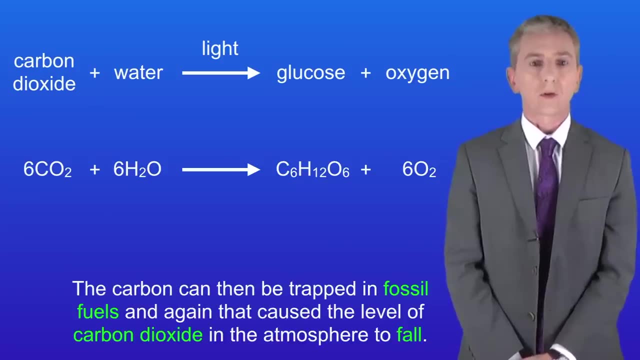 the equation of photosynthesis here. As you can see, as well as producing oxygen, photosynthesis also takes in carbon dioxide. The carbon can then be trapped in fossil fuels and again that caused the level of carbon dioxide to fall. So the level of carbon dioxide that 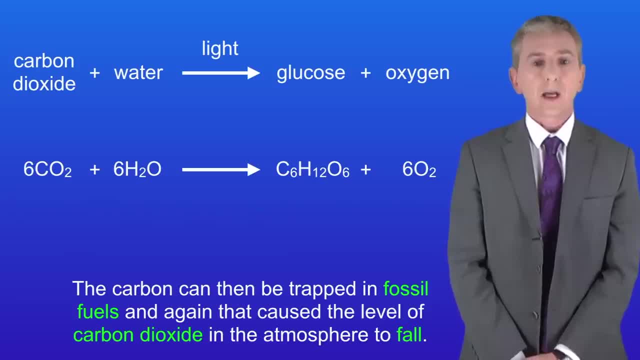 is in. the atmosphere has to fall and we'll be looking at how fossil fuels are formed in the next video. Remember, you'll find plenty of questions on the atmosphere in my vision workbook and you can get that by clicking on the link above. 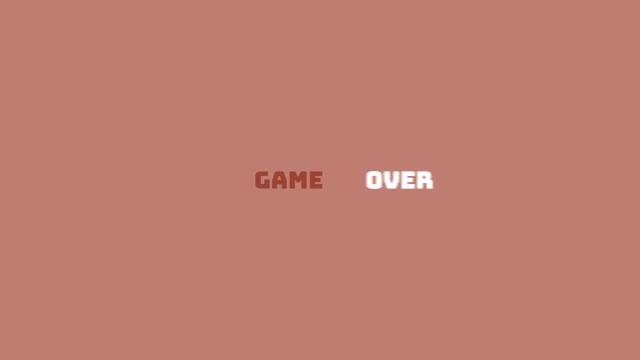 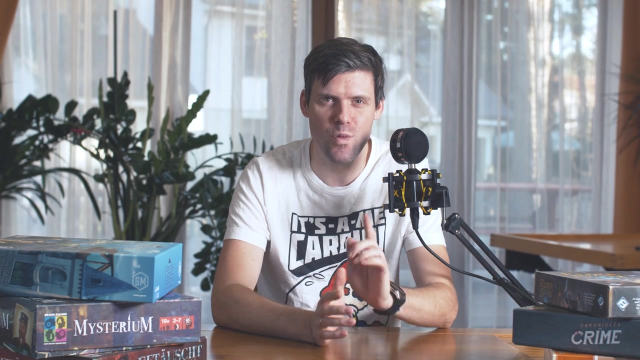 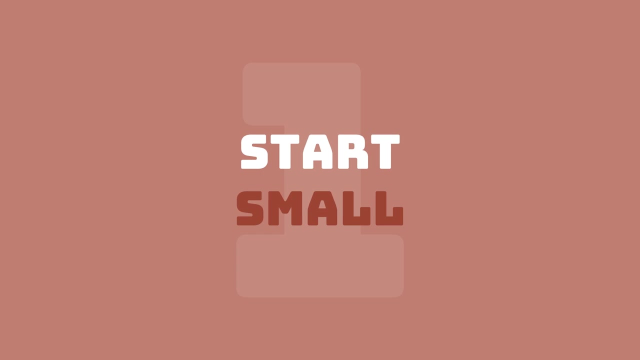 Hi, my name is Ioannis and welcome to Board Game Hangover. Today I'm gonna give you five tips that I feel have worked for me to turn my kids into real board gamers, not just some casual players like most are. Tip number one: Start small and make. 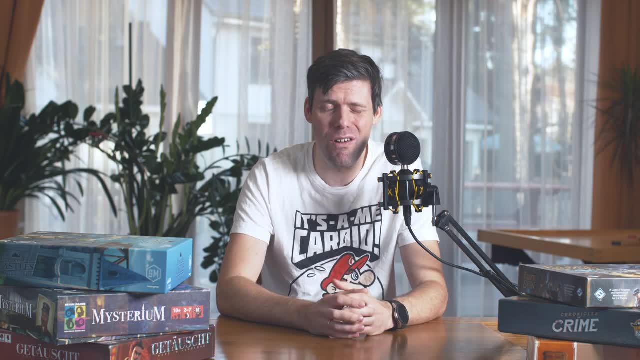 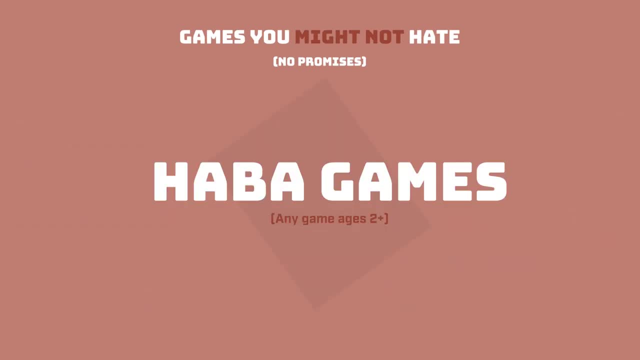 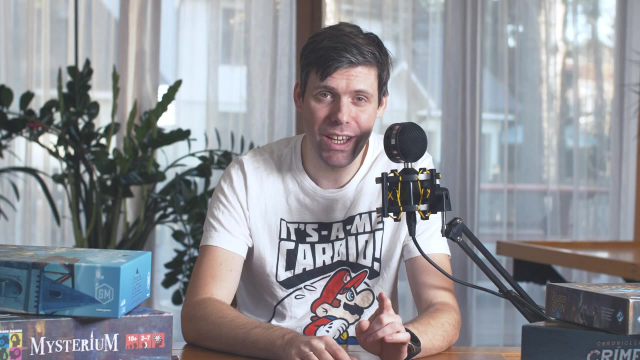 your way up. At the beginning you'll have to play all those boring games that you don't really want to play- Memory games or lotto or like simple, simple puzzle games. It's just something I know is super boring for you, but what it does for your kid- and it is an investment- is he will learn that. 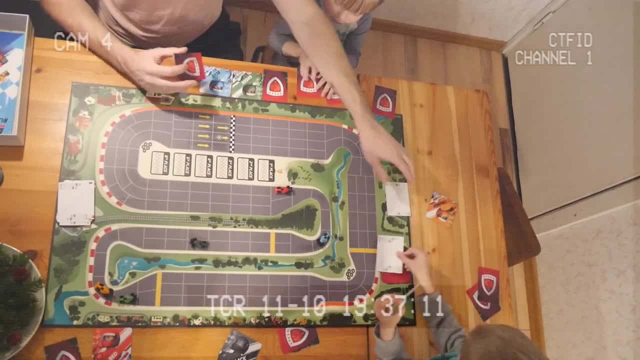 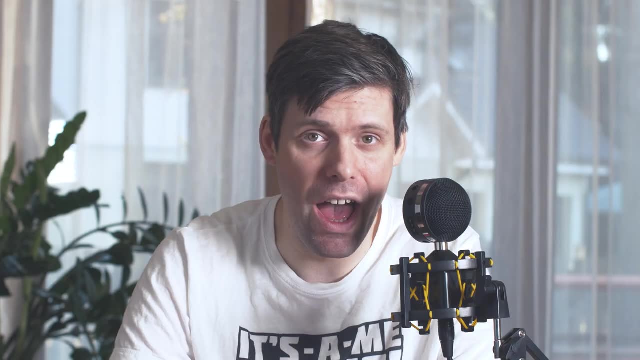 some things happen by specific rules and patterns. You can't start with something big immediately. It's probably gonna scare him off and he'll never play that Gloomhaven with you ever. Hey dad, I'm back from the kindergarten. Hi son, I know you're only five, but I got.